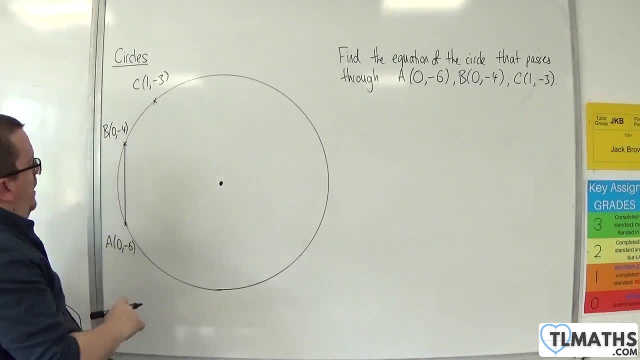 So first of all, I'm going to look at a and b. I'm going to find. well, because this is just a vertical line, it's relatively straightforward to find the perpendicular bisector, But I've got to find the midpoint And then, from the midpoint, draw my line. 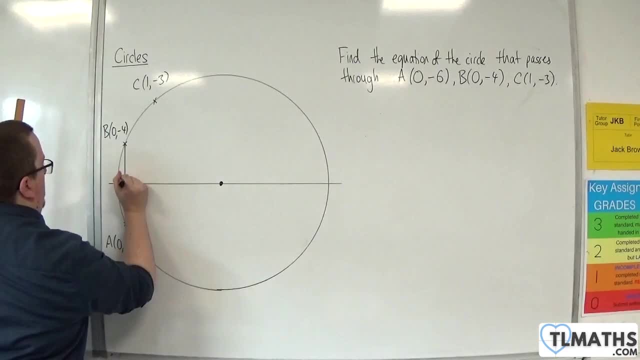 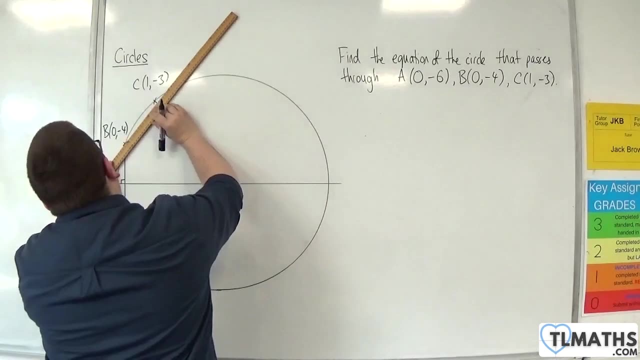 Okay, So that will be the perpendicular bisector of a and b, And then I'm going to find the perpendicular bisector, well, of b and c. Let's do b and c. It doesn't matter which pair I choose here. 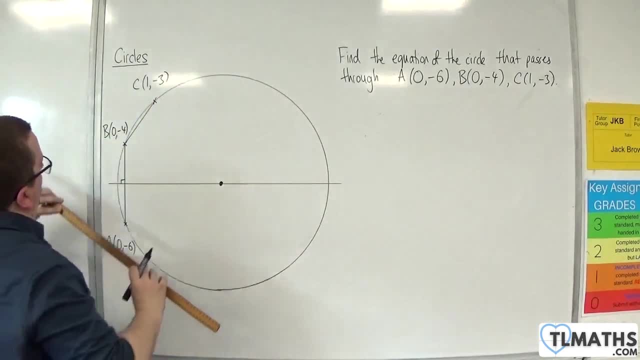 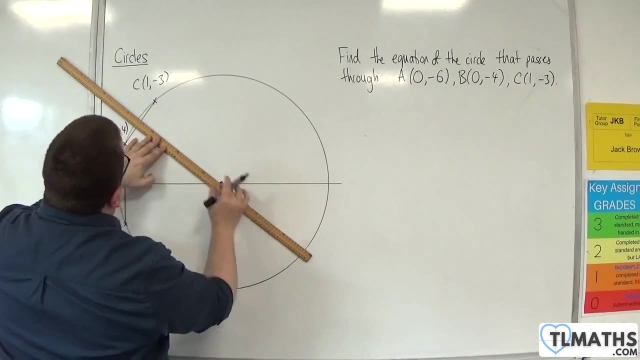 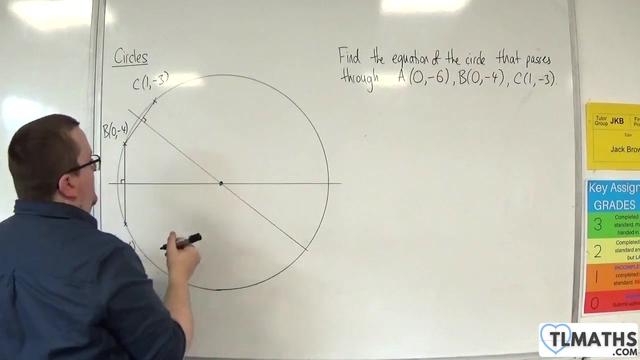 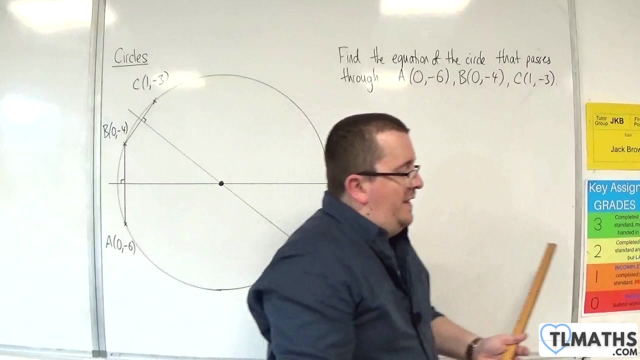 Okay, I'm just doing this because it's easier to visualise it. And then I find the midpoint, I find the perpendicular bisector And draw my line. Okay, so there's my perpendicular bisector, And you'll notice that both of those lines go through the origin. well, not the origin, sorry, the centre of the circle. 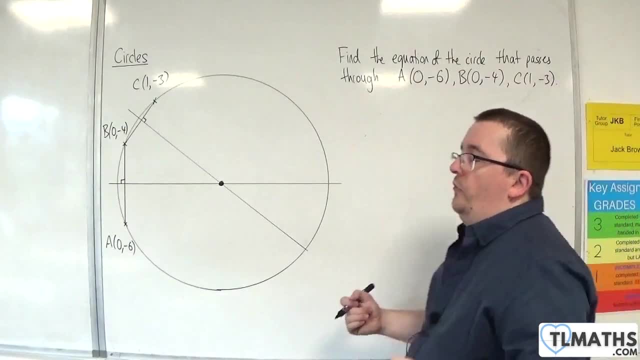 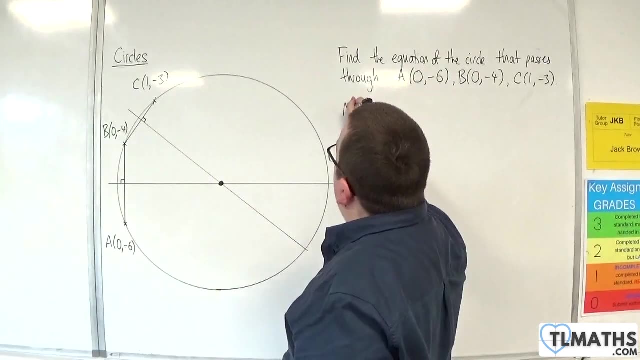 So this will happen. So this will happen Regardless of what circle you're dealing with. So if you've got three points, pair them up. So I'm going to be working with a and b first of all. 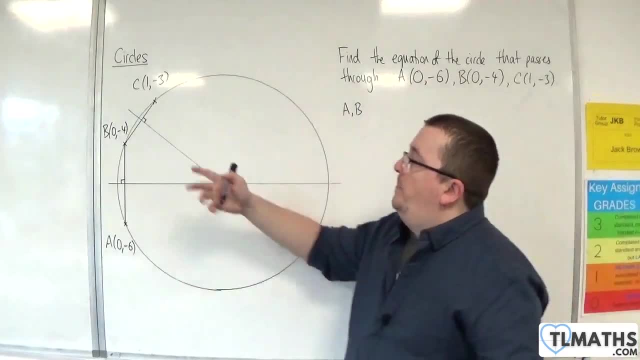 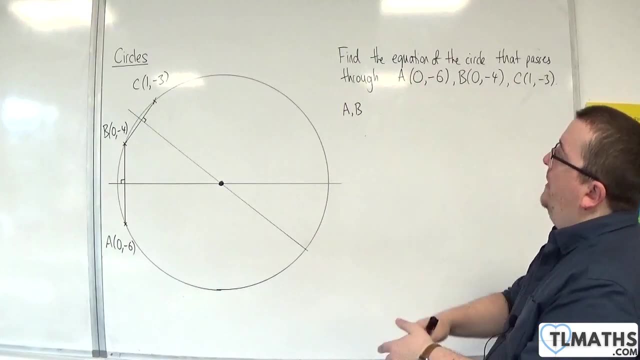 Work out the perpendicular bisector, Then pair up b and c Perpendicular bisector. Where those perpendicular bisectors intersect is the centre of the circle. Okay, And then I'm partway on my way to finding the equation. So let's work with a and b first. 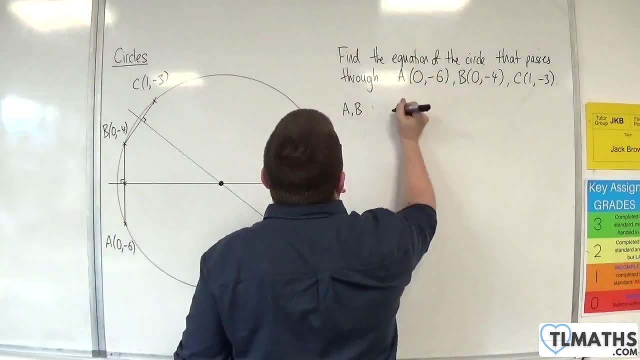 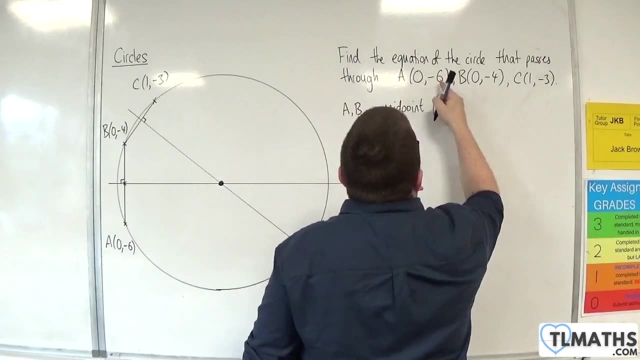 So first of all find the midpoint of a, b, So midpoint. So 0 plus 0 divided by 2 is 0.. Minus 6 plus minus 4 divided by 2 will be minus 5, of course. 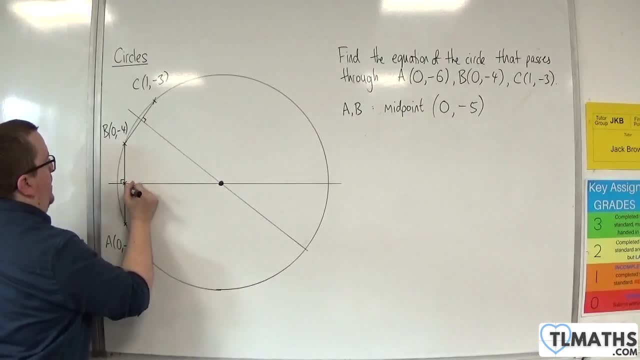 So this point here is going to be 0 minus 5.. Now the next thing I would do in general is find the gradient of this line, Then use the negative reciprocal. But because this is a vertical line, I know that it's just going to be a horizontal line. 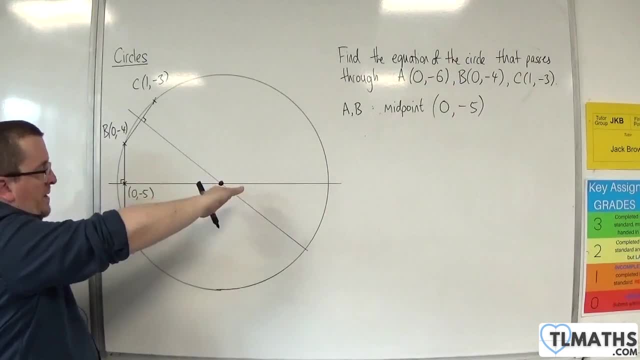 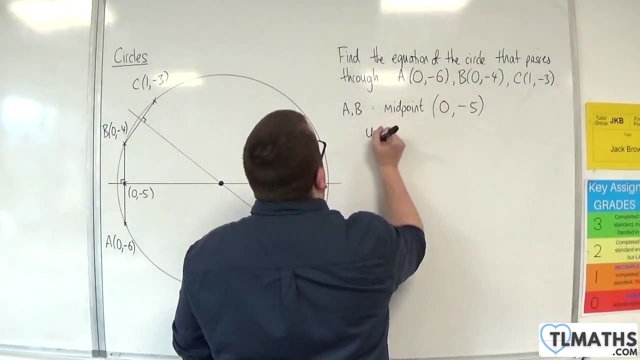 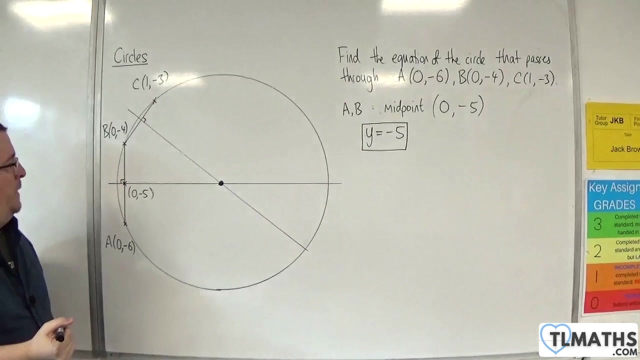 Okay for the negative. well, for the perpendicular bisector. So this line is just going to be: y equals minus 5.. So y equals minus 5 is what I want for that first one Okay. So that one's pretty straightforward to do. 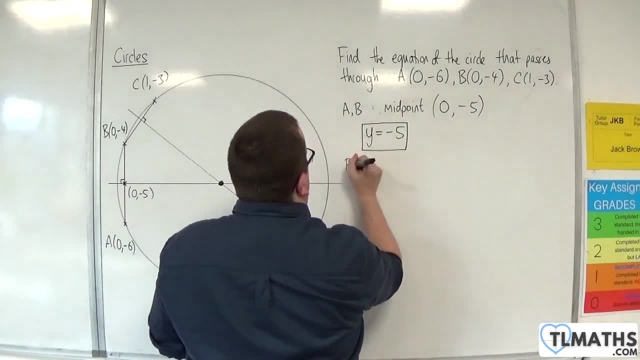 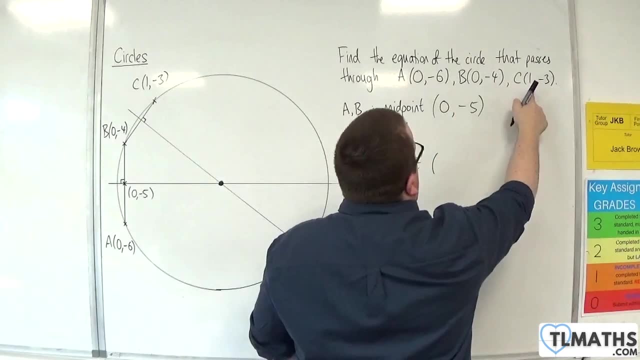 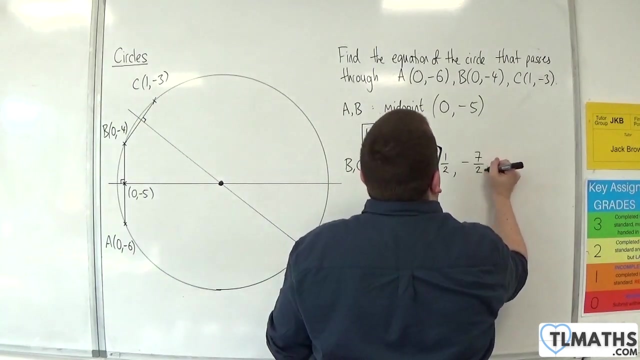 So now let's look at b and c. So midpoint first: 0 plus 1 divided by 2 is 1 half Minus 6.. Minus 4 plus minus 3 is minus 7.. Divided by 2 is minus 7 halves. 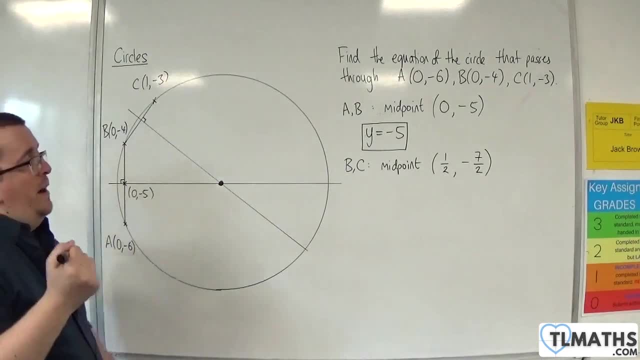 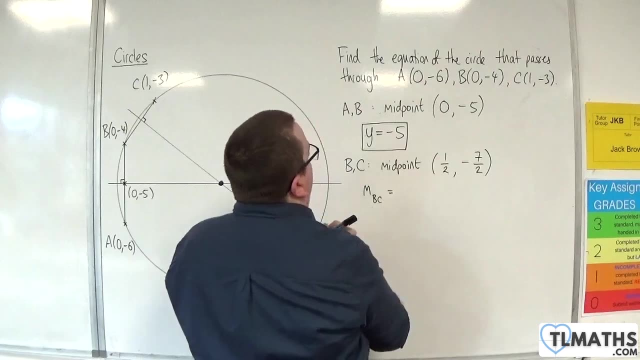 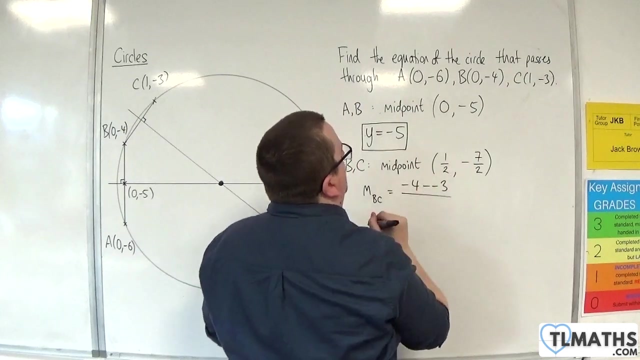 So we've got our midpoint. Now we need to work out the gradient between b and c. So the gradient of b- c is going to be the difference in the y coordinate. So minus 4, take away minus 3.. 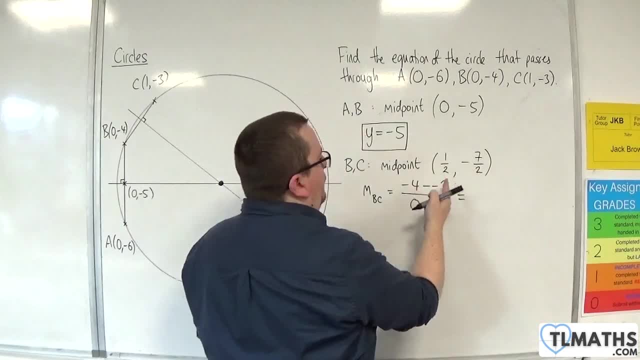 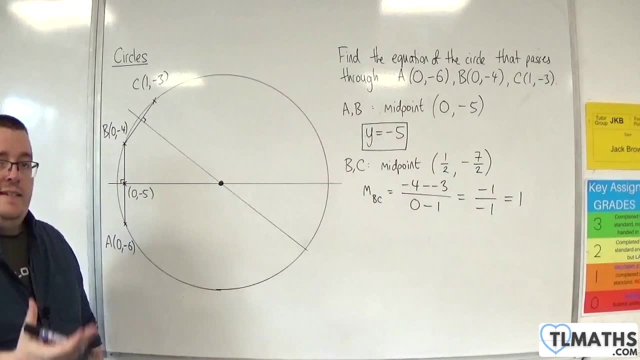 Divided by 0, take away 1.. So minus 4 plus 3 is minus 1.. Over minus 1. Of course that's just 1. So the negative reciprocal of that would just be minus 1.. 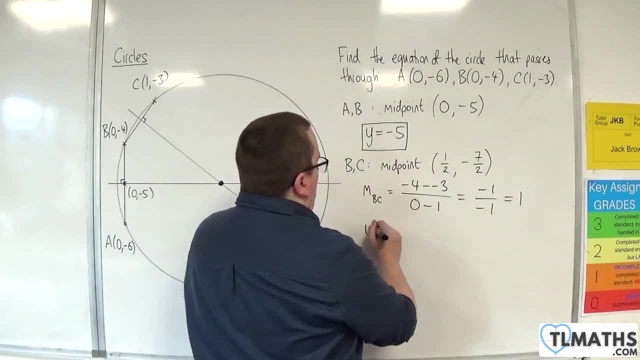 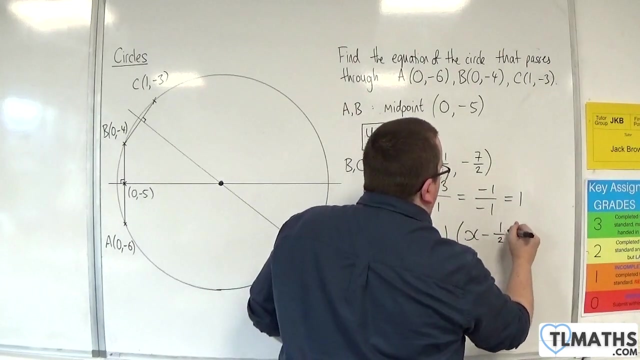 So the perpendicular bisector will be: y take away y1.. So plus 7 halves is equal to the gradient which is minus 1, times x take away x1.. So x take away 1 half. So this is the equation of the perpendicular bisector. 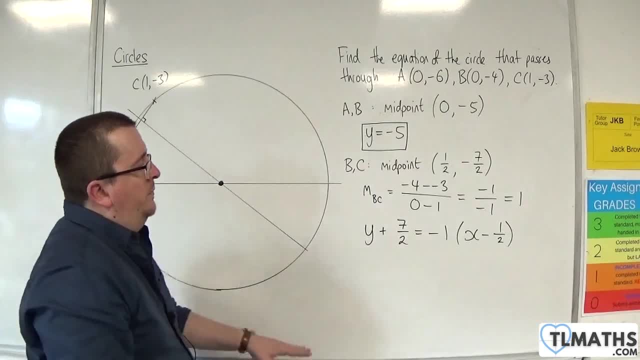 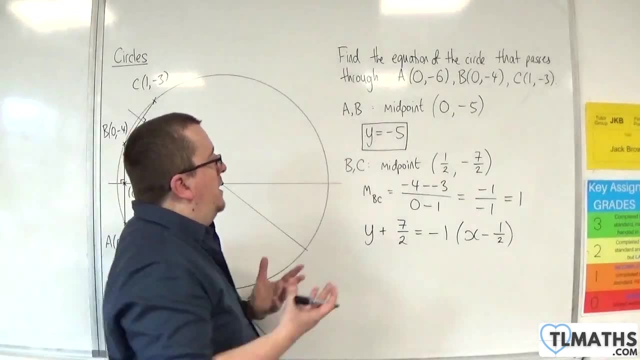 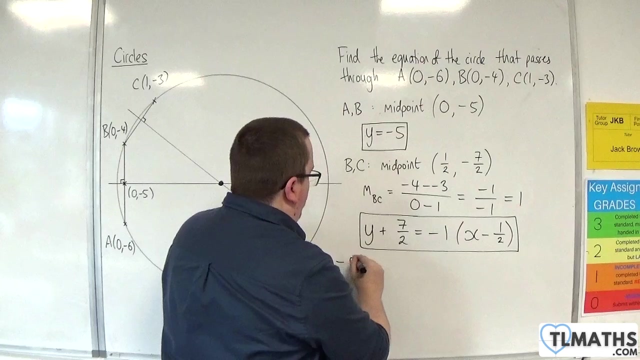 So that line there. Okay. So what I can then do is- I don't need to rearrange this into any other form- I can just substitute y equals minus 5 into this. So minus 5 plus 7 halves is equal to minus 1 times this. 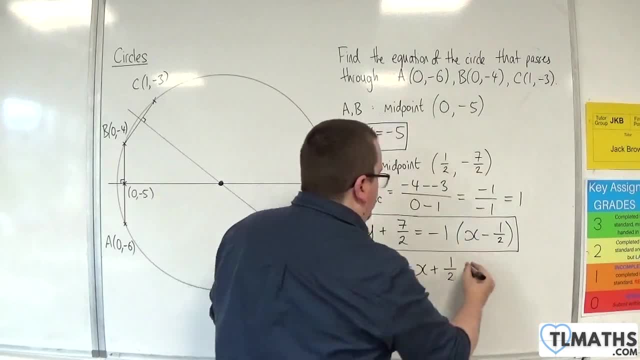 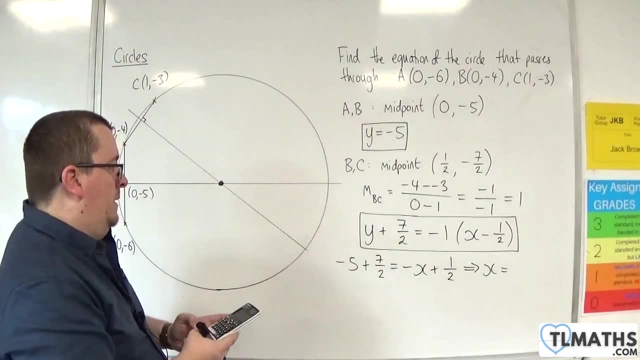 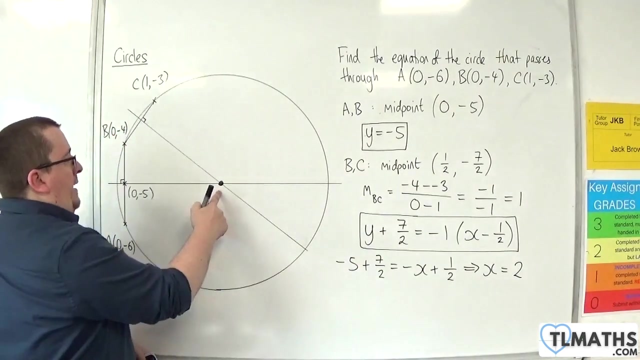 So minus x plus 1 half. Okay, So minus 5 plus 7 halves. take away a half And then it's the negative of that, So that would be 2.. So this point here is 2 minus 5.. 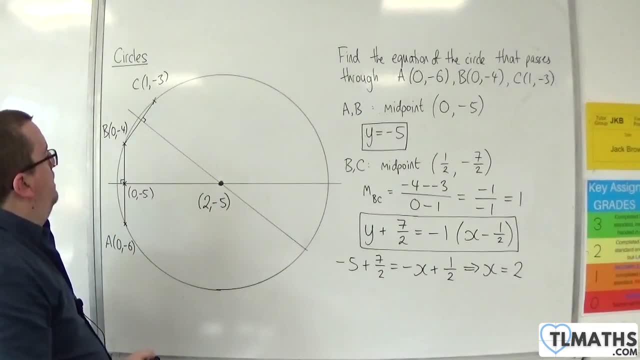 So I've now found the centre of my circle. The next thing I need to do is I need to work out the radius of the circle. Now, to do this, you just need to choose any of your points that you want, Any of your points that you know that lie on the circle.